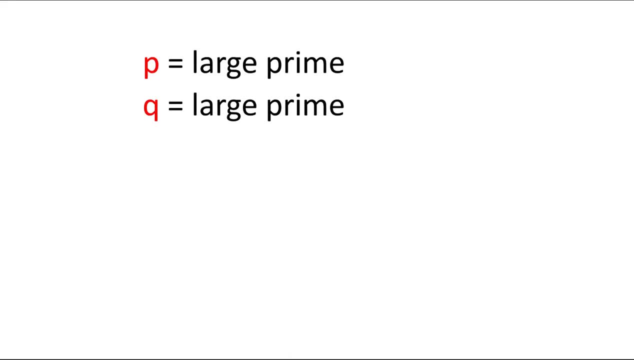 and q, which is exactly the same. These are normally randomly generated, just really big numbers, And we've got n, which is p times q, r, which is p minus 1 times q minus 1, e. This is typically just a fixed value. So, yeah, this is something that I struggled with to start with. 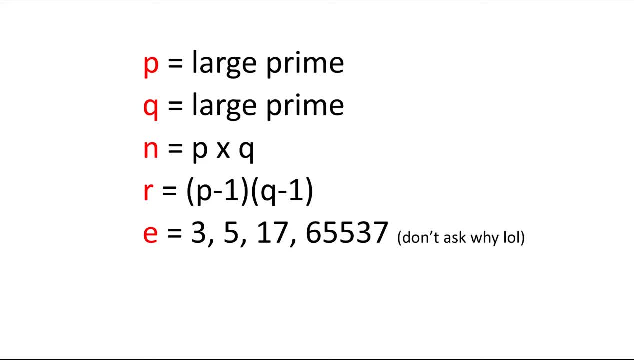 because I couldn't figure out how people got to e. but really you just need to use one of these four numbers. So remember those. you can write them down or whatever, And normally it's the bigger the value of e, the bigger the value of q. So you can write them down or whatever, And normally it's the bigger the value of e. 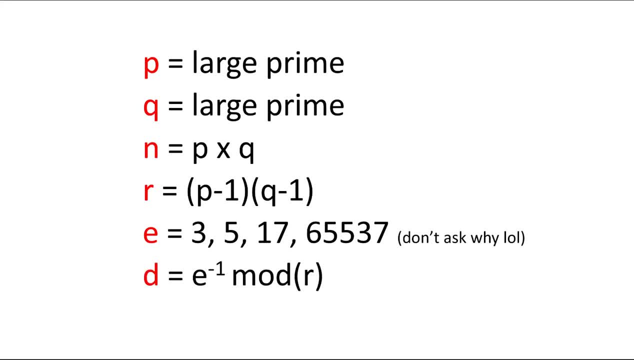 the more secure the algorithm. And d, which is e minus 1 mod r, and we'll talk about that in just a second. And just as a little note, I've sometimes seen r called phi, denoted by that symbol there, or the totient of n. So if you see any of those, they're just talking about r. 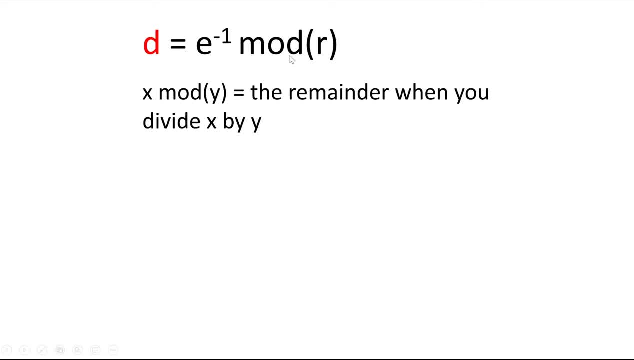 All right. next we're going to look at modulus, so what this mod r actually means, And it's pretty easy. it's just another thing that confused me Back in the day, so I'll clear that up for a second. It's literally just the remainder. 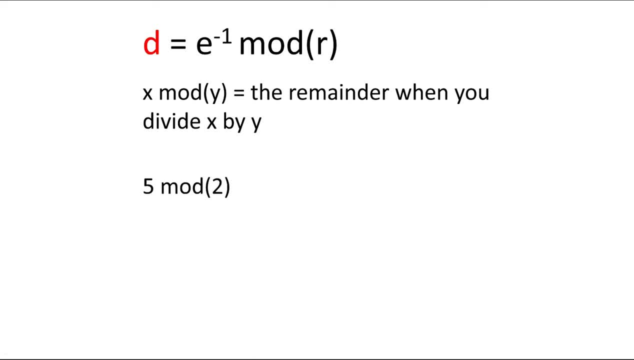 when you divide x by y. So if you have 5 mod 2, it just means you divide 5 by 2, which gives you 2, remainder 1.. And then the answer to 5 mod 2 is just 1,. 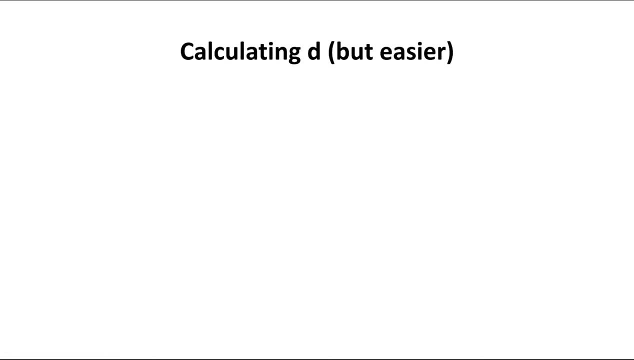 it's the remainder of that calculation. All right, I've seen, I mean everywhere, people use the Euclidean algorithm to find d, but the fact is there's no situation you're ever going to need to calculate d by hand, right? you're always going to have a calculator with you. 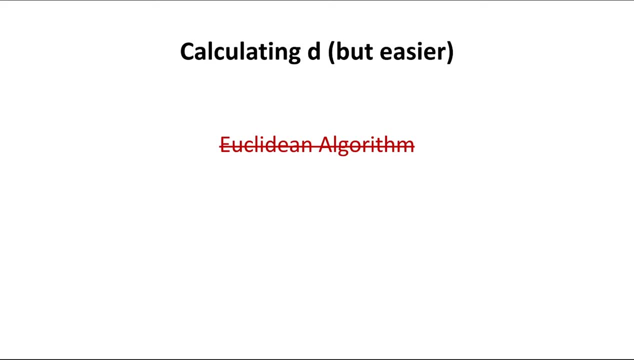 Like for my exams I had a calculator, but I never had to do this, so I'm not going to worry about teaching that, But I might do a video in the future with it and we'll just see how it goes. But I've literally never had to use the Euclidean algorithm. 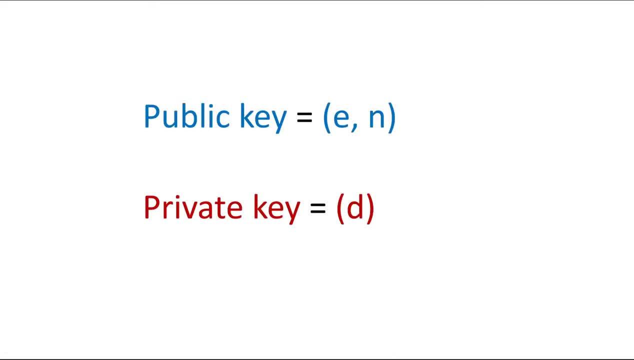 so I just wouldn't worry about it for now. right, so we've got the public key, which is the e and values we found before. that's what's put to the public, everyone knows it and that doesn't affect the security of the algorithm. and then you've got the private key, which is d, and that's what you. 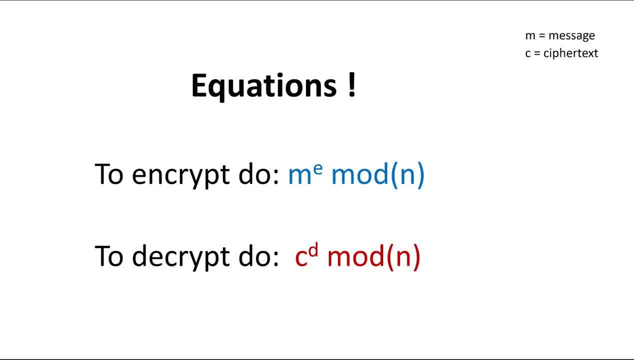 don't show anyone. that's what you keep to yourself. and now on to some equations. these are to, obviously, to encrypt and decrypt messages using RSA, and it's really easy. you just got m to the e mod n, so that's the message to the power of e value from earlier mod n, which is the p times q value we have. 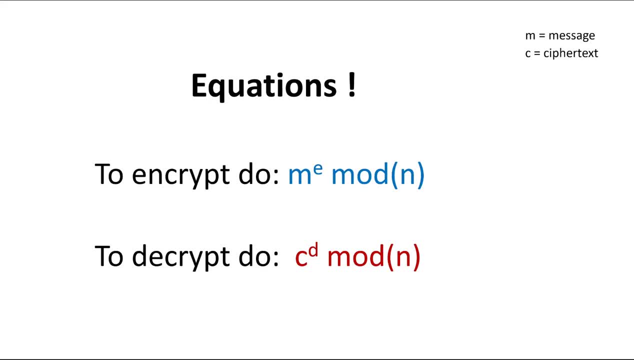 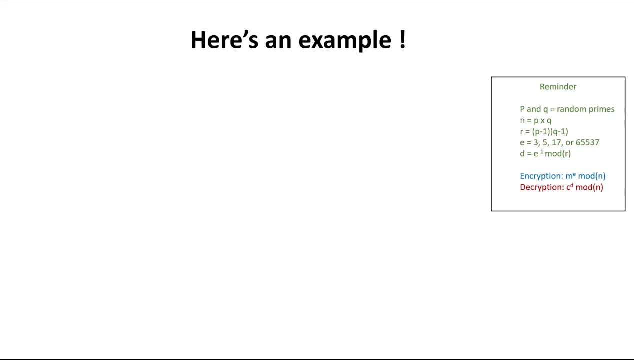 and then to decrypt, you got c, which is the ciphertext to the power of d, our private key, modulus n as well. all right, so now we're going to do an example for encrypting and decrypting with RSA. I've got a little reminder on the right there. 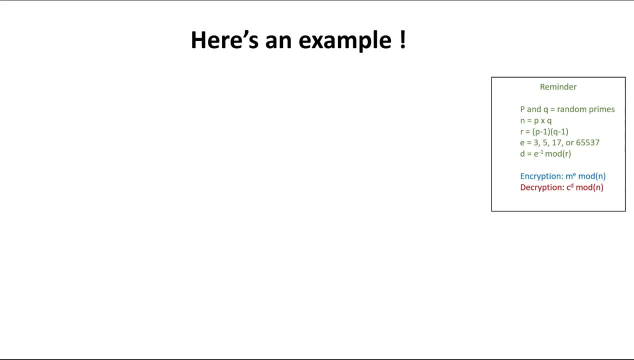 of how we got to all the values. this thing refer back to it. all right, so we got p, which is 11, it's just a prime number, and q, which is 3- it's just another randomly chosen small prime number, and n, which, as you can see, is p times q. 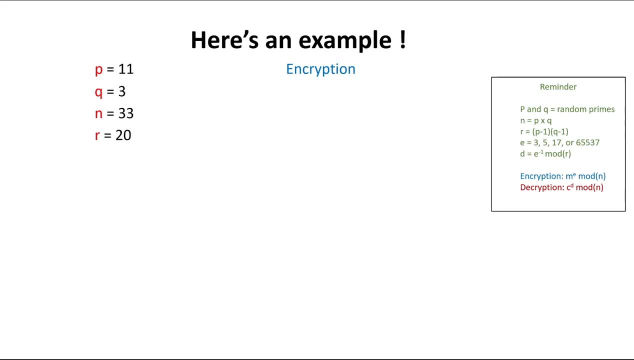 33, and r, which is p minus 1 times q minus 1, which is 10 times 2 in this case. so we've got 20 and e. we've picked the smallest value from the options earlier, just to make it easier, which is 3, and d equals 7. like I said, I'm not going to go over Euclidean algorithm in this video. 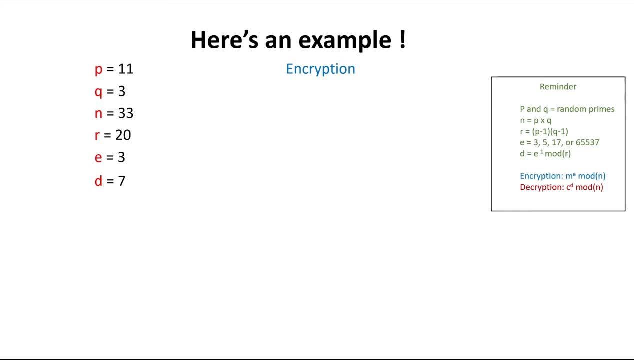 you can just plug our values into a calculator, right? so I'm going to go over Euclidean algorithm in this video and I'm going to go over the values. so in this example we've got our message, which we can. we've just got 7 for our value. 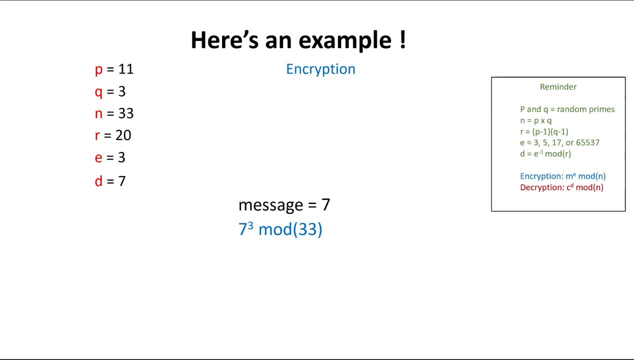 and to encrypt. we'll do 7 to the 3 mod 33, which, if you look in the right there for encryption, it's our message. so the power of e mod n 7 to the power 3 is 343, 343 divided by 33.